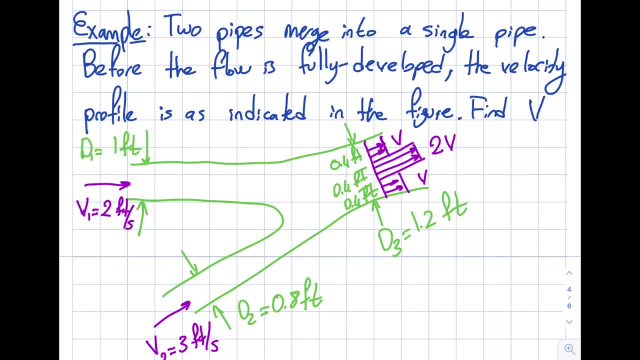 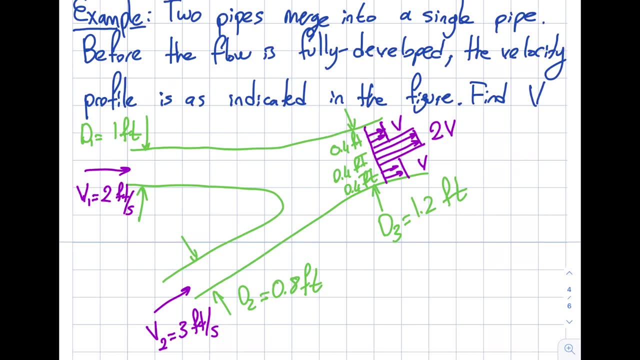 given as one foot. the last one is two feet per second. the velocity two is three feet per second. diameter two is 0.8 feet and over here- this is the tricky part, let's be careful over here. so this entire diameter is 1.2, okay, and the central is: 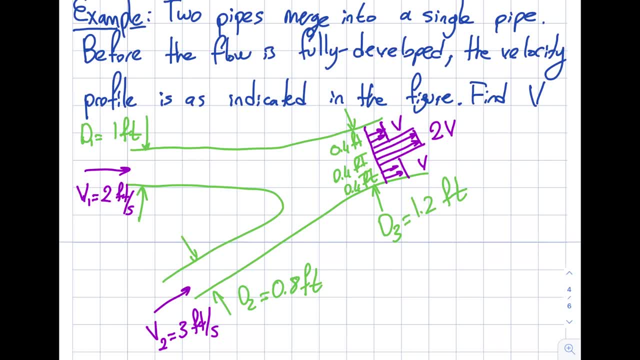 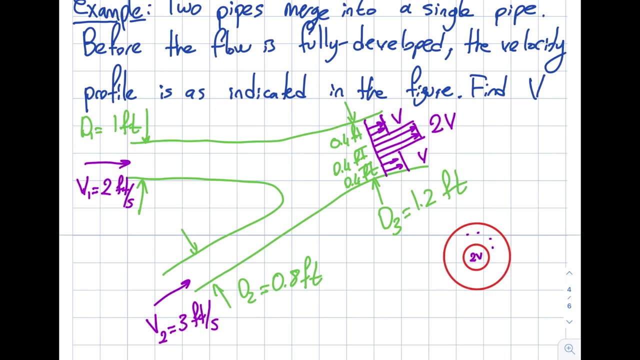 0.4 foot diameter section has a velocity of 2v and the remaining of that will have the velocity of v. so i want to actually go ahead and plot this so that we are on the same page. this section is 2v, the outside that i have here is v. so i'm looking this direction over here. okay, do you? 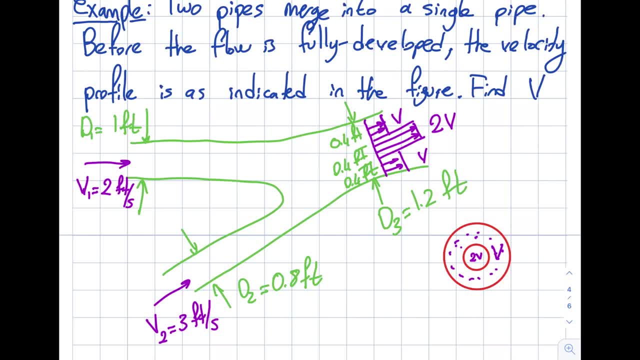 see what what it is. so 2v is at the central and the diameter to here this is 0.4. the central section and the whole thing from here to all the way to here is 1.2 feet. i will establish steps um after the module sex, because things are going to get more complicated. 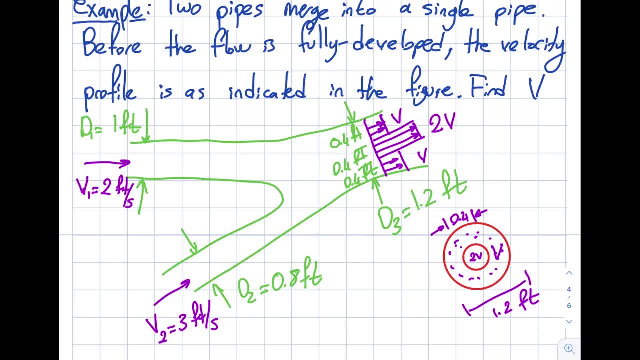 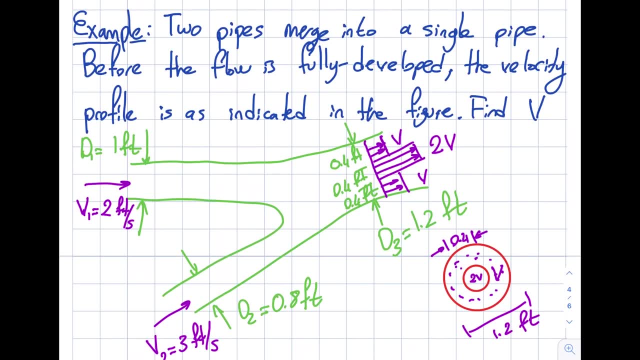 and i would like you to clearly follow the steps. but it's never too early to start. the first step is to read the question. you'll see. you look at the question, you read the question. it's a dumb step for now because i'm reading the question, solving the question for you what i expect you. 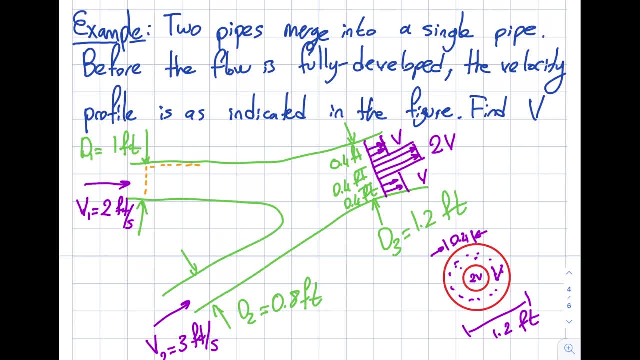 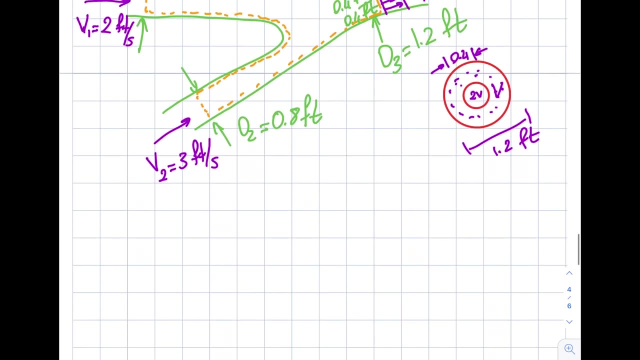 to do is to do is to solve the question. so i'm going to write down the assumption in the course and i'm going to see you write down the same steps two. so now this is the same step, and then let's just listen to the question. i have read this way. it is writing a very clearly as this: 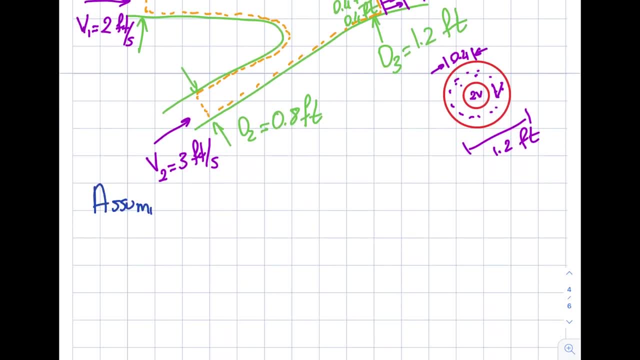 is a pleasant question. so the first step is to take into account the significance of the question and the second step but you know that you can think of it as a solution. so this is a serious question and we're going to take it right away. and then we're going to take into account the 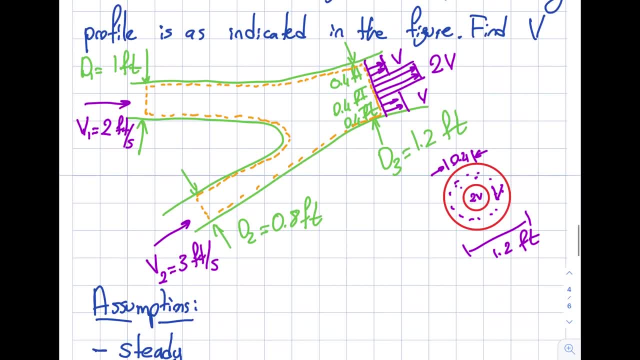 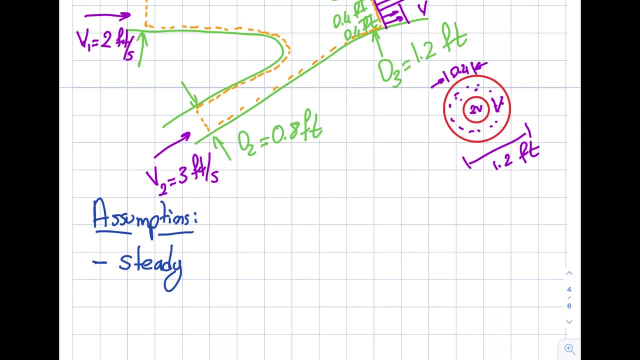 dependence in the question. no, so that's the reason. okay, i don't see anything related to time. if i head over here, let's say that in section number two my v2 is three feet per second plus 0.1 t, then it will be unsteady flow, okay. second is: is this constant density? yeah, i can't say that. 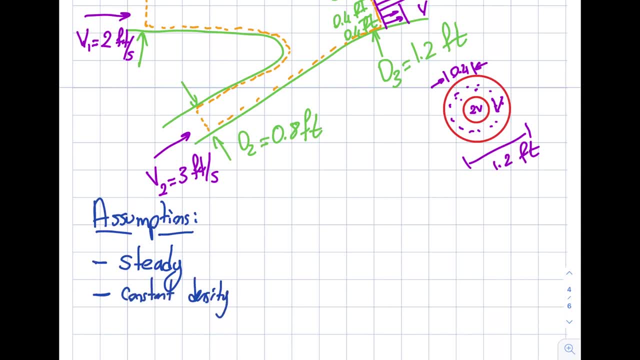 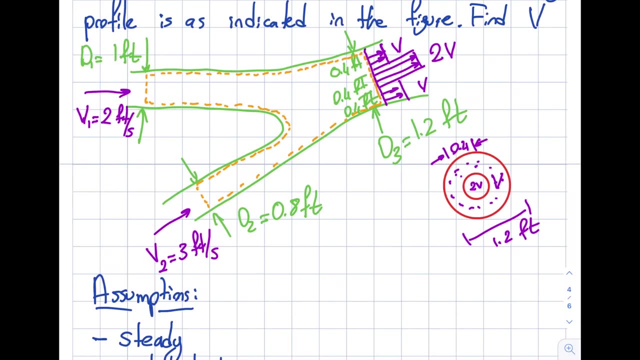 because this is water liquids. it's a good assumption to have constant density for gases. you need to be careful. and is this uniform flow? so, if you follow what the numbers recommend you, the answer is one: section one and section two. yes, section three is no. okay, so i have to deal. 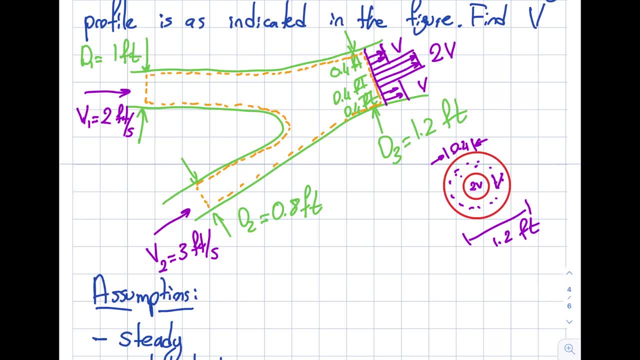 with this integral formula, which i don't really like. so what i'm going to do is- this is a trick that i would like you to know- i'm going to separate the section three into two separate parts at the center of this. let's call: right over here. i'm going to call: this is section four, and 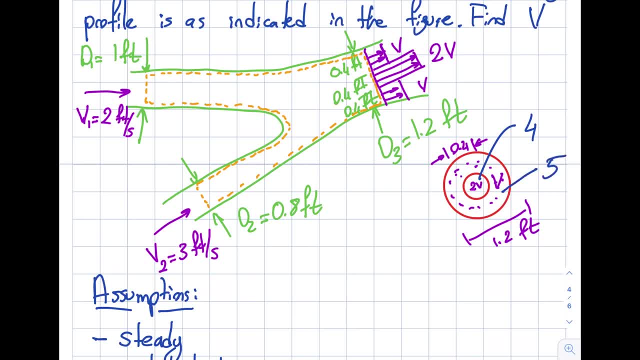 the remaining of this, i'm going to call this section number five. my goal is to ensure that over here it's exit four. i have a uniform velocity. the loss is not changing. at section number five, the velocity is also not changing. it's different than four, but it's not changing. 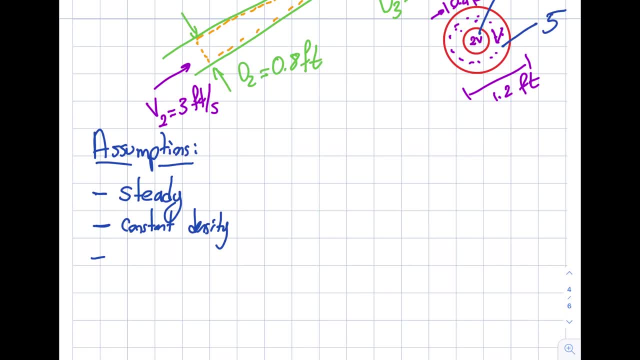 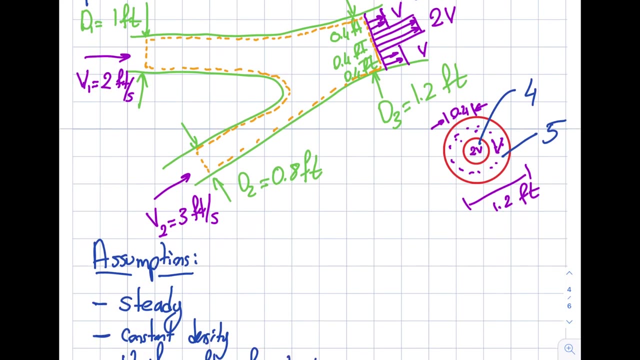 so now i can go ahead and say that uniform flow i'm gonna, you know, like four, one, two, four, five, just to be clear. the next question is what happens to my conservation of mass in this particular case? so i'm going to call this section four and 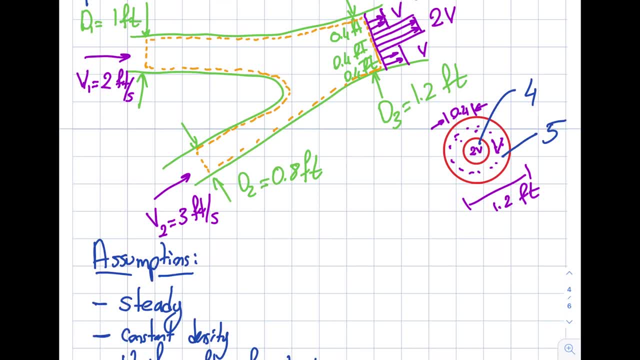 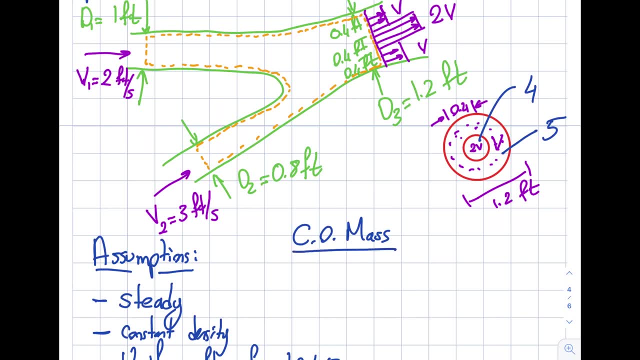 let's go ahead and write it. it's going to be conservation mass and let's go ahead and write this. so it's going to be summation over the inlets v in net and i may have called this vni. ai will be equal to exits v, exit a exit. okay, you can call this ni and any, it doesn't really matter. 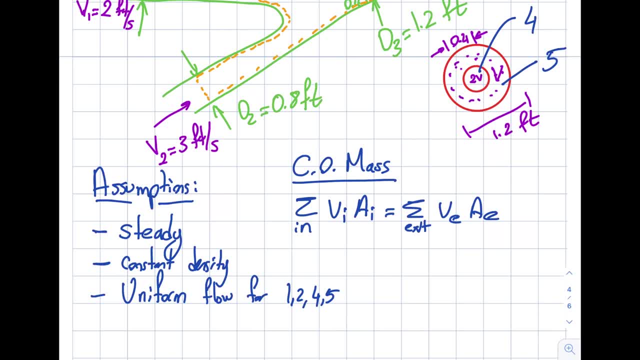 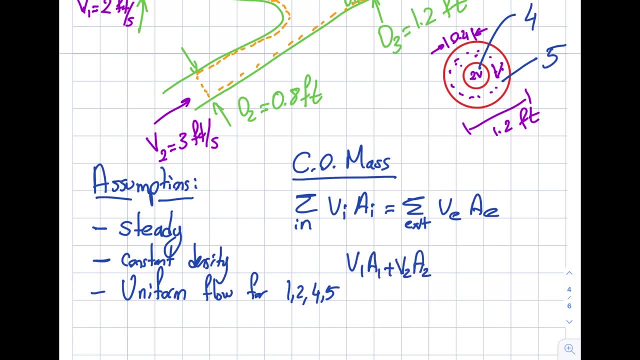 so let's look at the inlets. so the two and one, those are the inlets. so then this will become like this: v1a1 plus v2a2. so far, so good. how about the exits? remember that i separated it into two over here, so it's going to. 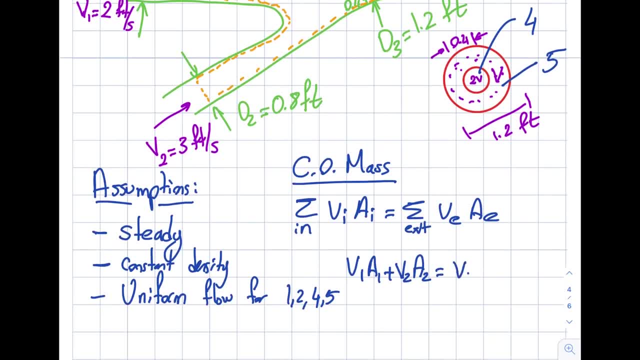 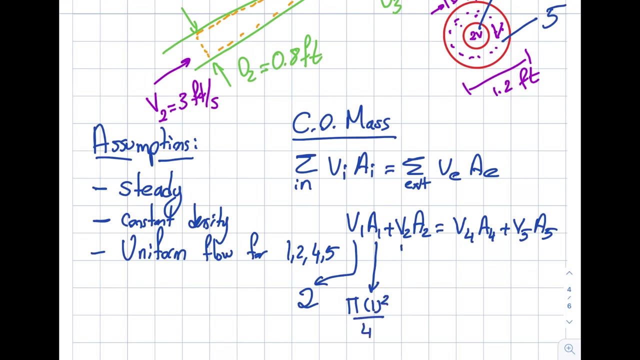 be four and five, so let's write this: v4a4 plus v5a5. simply, i go ahead and write my numbers in, so let's go over here. v1 is two- i can see barely over there right. a1 is- i think it was one, right? yeah, uh, pi one squared divided by four. v2 is right over there. 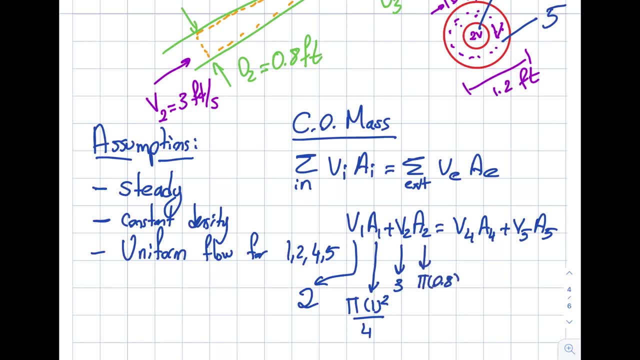 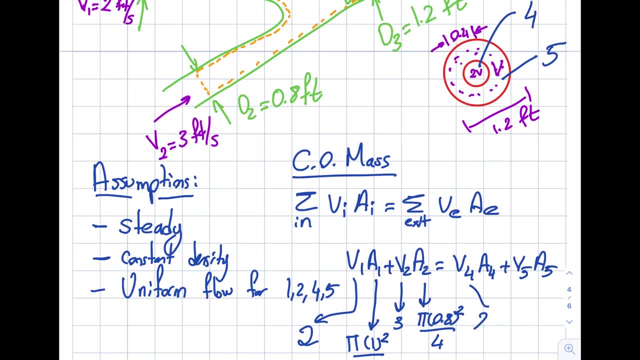 it's three. a2 is pi 0.8 squared divided by four. v4- four is the central region, so that's two v. what about a4? that is going to be pi 0.4 squared over four. right, so that part is easy. how about v5? so v5 is v. that's given to me, okay, so 2v is for the section. 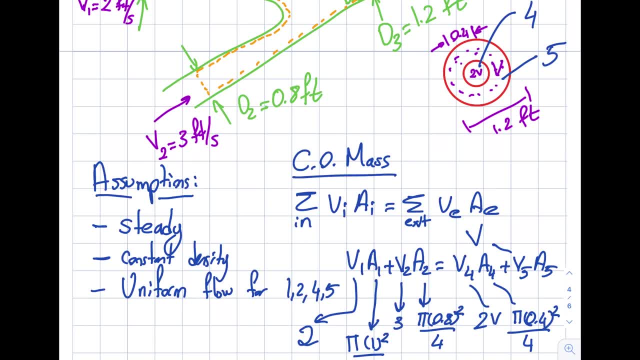 4 v is for section 5. what about the area 5? it will be the entire area of the circle minus this interior one. so think of this as like a donut, right? so this is the region that you eat, right? so i'm gonna take this entire area minus this area. that will leave me what i need over here. 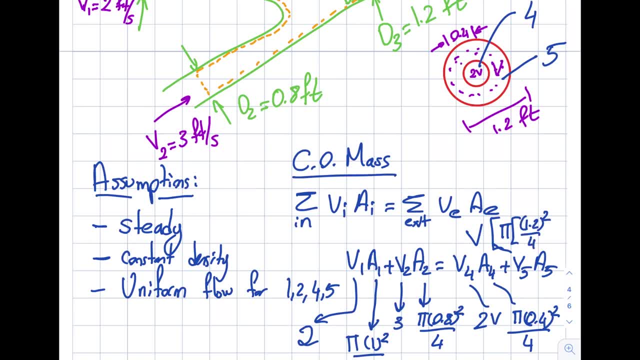 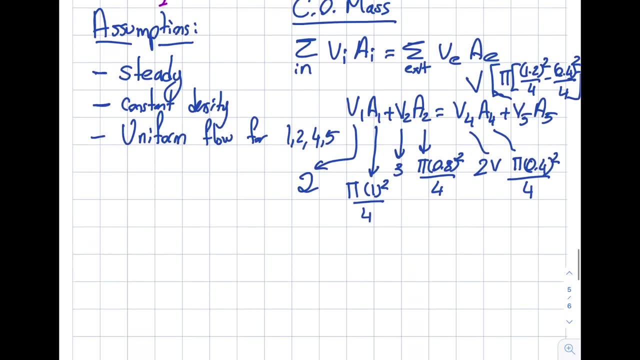 pi 1.2 squared divided by 4, minus 0.4 squared divided by 4, and i close the bracket. so let's just write this nicely so 2 times. first thing is, i will cancel the pi's. do you see it? every term. 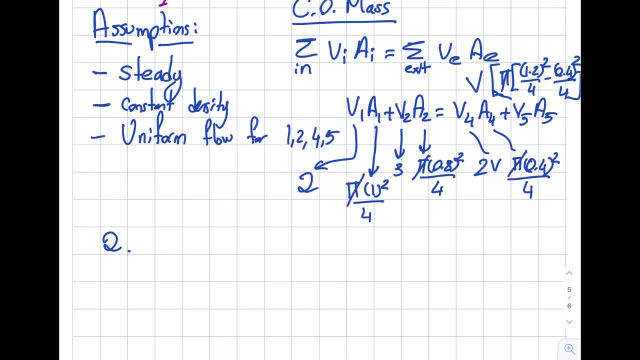 is multiplied by pi's, so i don't want to rewrite this. so it's going to be 2: 1 squared over 4 plus 3: 0.8 squared divided by 4 will be equal to 2v 0.4 squared divided by 4 plus v times. okay, this is a 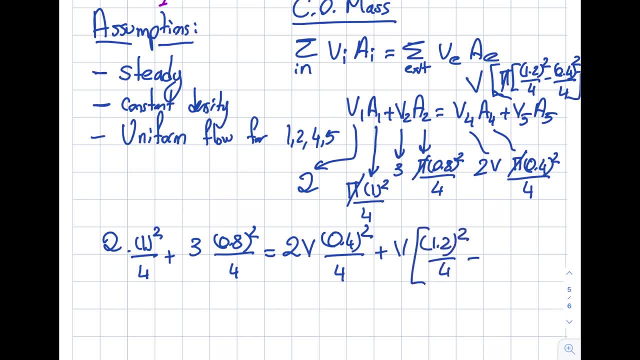 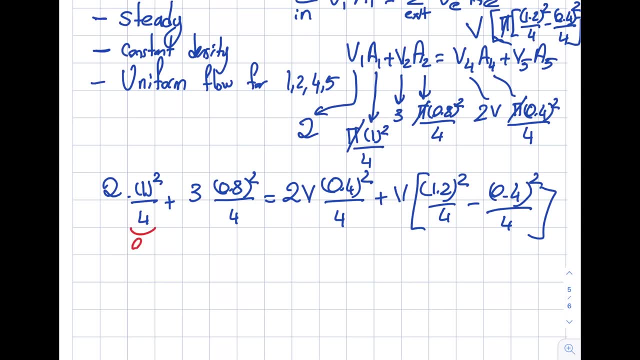 bit tricky: 1.2 squared divided by 4 minus 0.4 squared divided by 4. so this becomes to me: this is 0.25, right? how about this? this becomes 0.8 times 0.8 is 0.64. 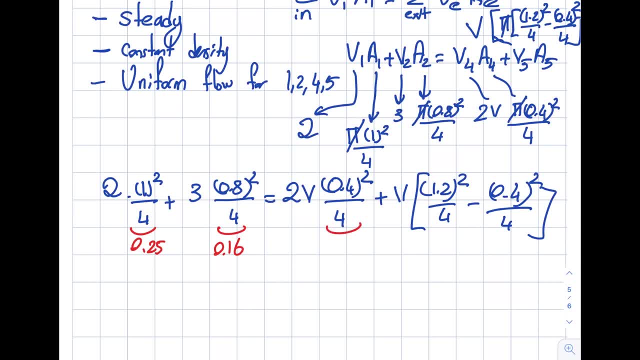 divided by 4 is 0.16, 0.4 times 0.4. divided by 4 is 0.04. right, and how about here? so 1.2 squared is 1.44 minus 0. point 16: one point two. eight point two. eight divided by four is zero point.